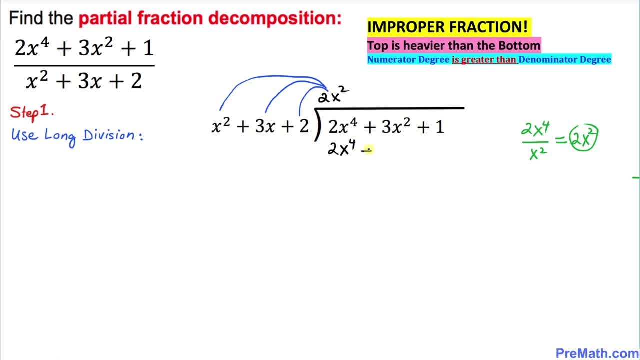 times 3x. This 3x is going to become 8x, 3x plus 6x, power 3 and plus 4x square. So that's the very first step. Let's go ahead and change the sign said the side. So this up. 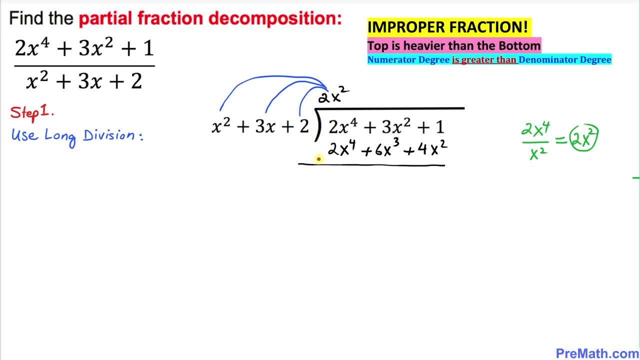 2x power 4 has a positive side. We're going to switch it to negative. This positive becomes negative as well, and then 4x squared, This positive sign is going to become negative as well, and as we can see this- 2x power 4 and minus 2x power 4- they are gone. so I can write. 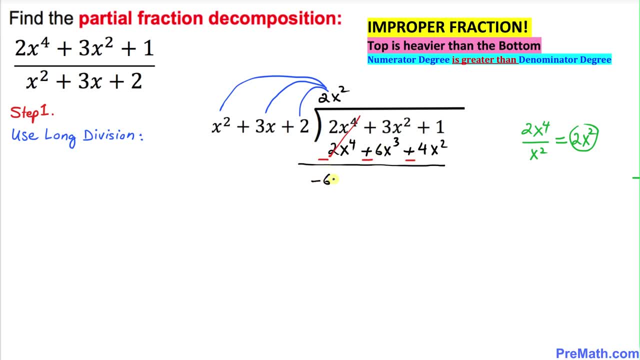 this as negative 6x, power 3 and, as you can see, this 3x square and negative 4x square is going to give us negative x square, and we are going to bring this one down over here become positive 1. now let's go ahead and repeat the same process once again. this, the leading term, is: 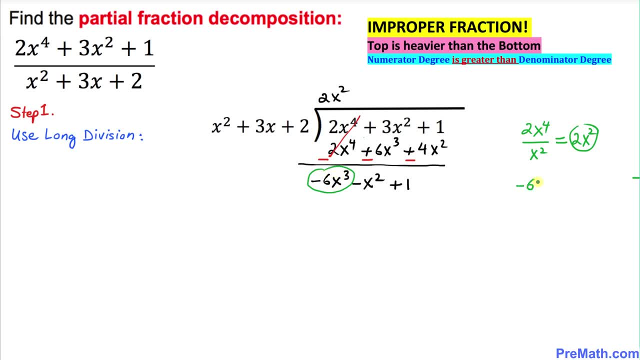 negative 6x power 3- I can write it over here: divided by the leading term on the outside, this divide by the value 6. shit, this is the horizontal power and that is negative 6x power 3. over here, divisor is x squared. let's go ahead and simplify this thing. that's going to give us negative 6x. 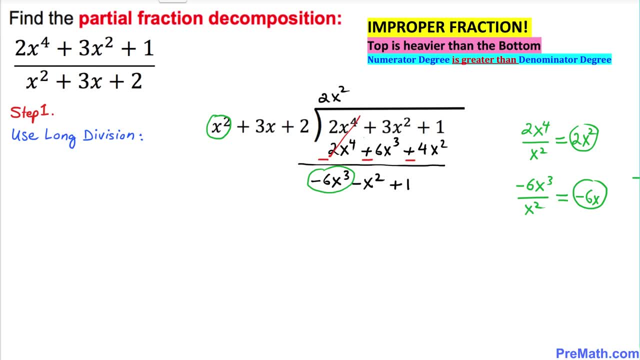 so we are going to write down this negative 6x on the top and we are going to multiply this negative 6x. we are going to distribute once again with all these terms. so let's distribute this thing: negative 6x times x squared is going to give us negative 6x power 3, and then it's going to become: 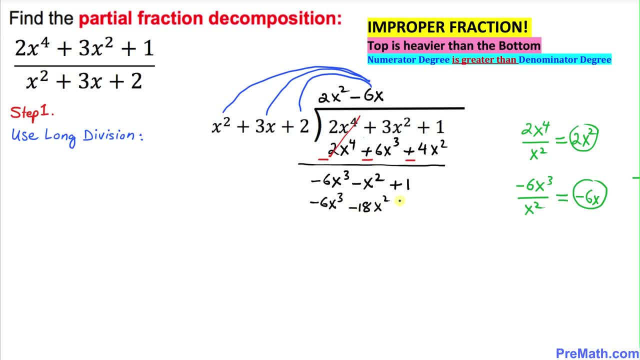 negative 18x squared, and then minus 12x. and once again, we are going to change the sign. this negative is going to become positive. this negative become positive as well. and over here, this negative become positive. you again, all right. so let's simplify this one, as we can see that this negative 3x, 6x squared, rather, 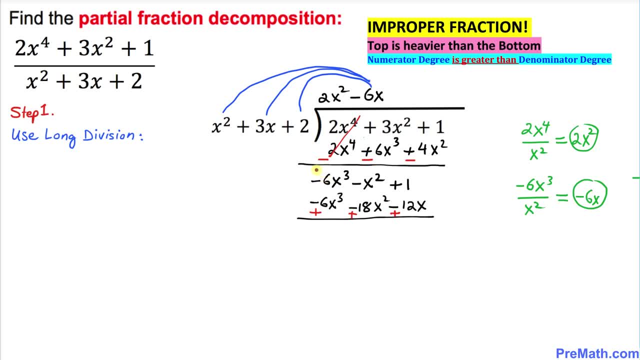 and this positive 6x squared. they are gone, as we can see. and here we got positive 17x squared and this is positive 12x, and now we are going to bring this positive 1x and this is positive 12x. and now we are going to bring this positive 1x and this is positive. 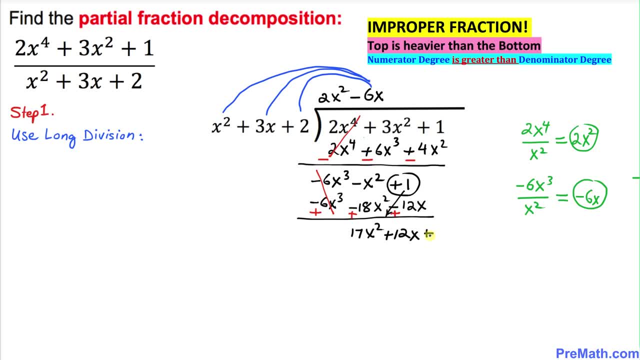 1 down over here, so that's going to become positive 1. now let's do once again. look at this leading term over here, which is 17x squared divided by. let's look at this leading term on the divisor, which is x squared, and when we simplify that is that's going to give us. 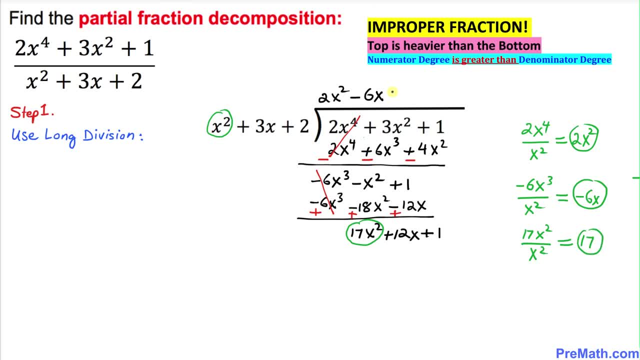 positive 17x squared. and when we simplify, that is that's going to give us positive 17x squared. and when we simplify, that is that's going to give us positive 17x squared. and when we simplify, that is that's going to give us. 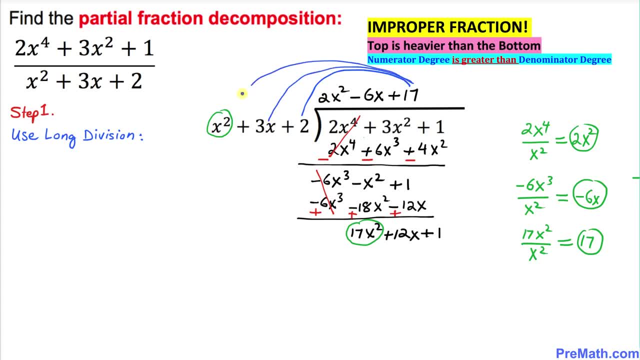 1xx squared and't then plus 15x squared once again and we get plus 34. let's go ahead and change the sign once again. this positive become negative, positive become negative again and this positive become negative. so we are going to cancel this one out. 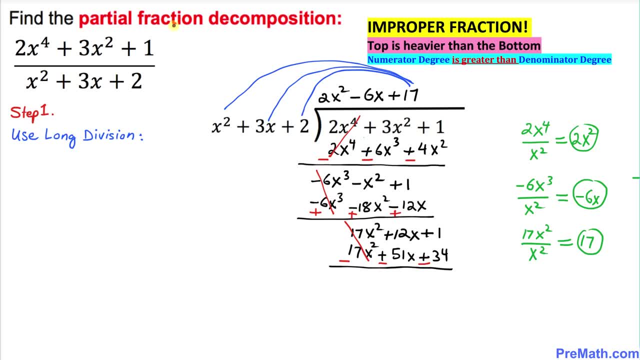 as we can see that they have a different signs, and this could be written as negative 39 x minus 33. so thus our remainder is negative 39 x minus 33 and, as you can see, the degree in this remainder is less than the degree of this divisor. so we are going to stop at this point. 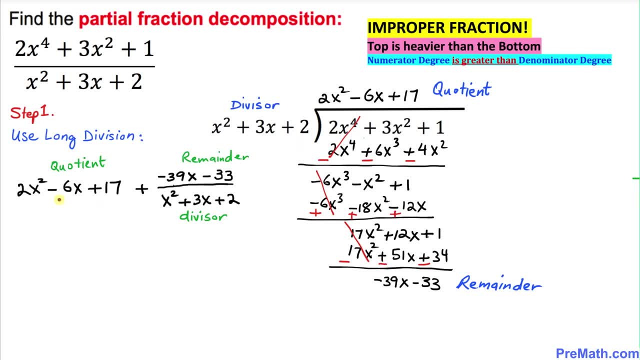 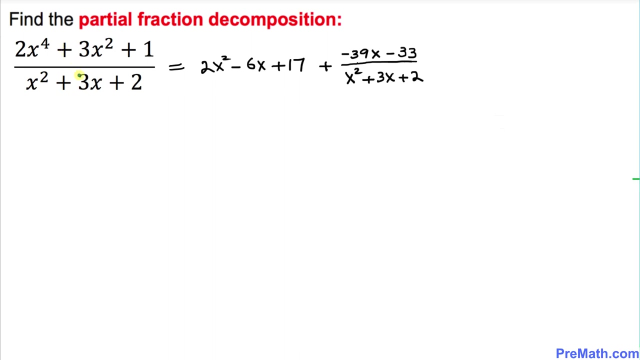 so thus we can write this as this one over here: 2 x square minus 6 x plus 17, is this our quotient. and then we always put a plus sign and this is our remainder and this the denominator. we have our divisor. so now we can write this our improper fraction. 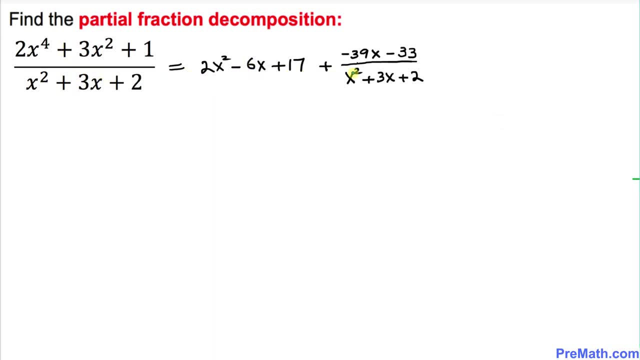 after long division, we can write it as this one: now let's focus on this part, this fraction. this is indeed a proper fraction and we will find the partial fraction decomposition of this fraction. so in our next step, we are going to find the partial fraction decomposition of this part, which I have just copied down over here. and if we look at this fraction, 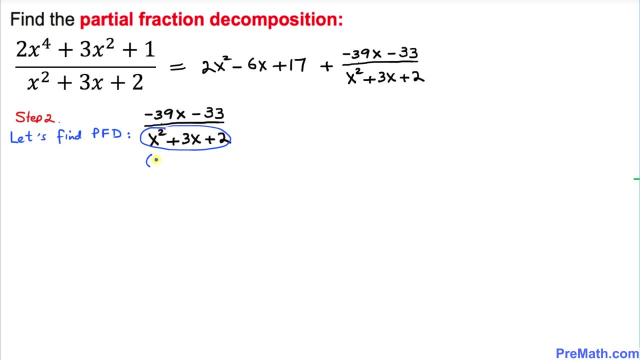 this denominator could be easily factored out into x plus one times x plus one times this particular fraction which we have just copied down over here, plus two. so therefore this fraction could be written as like this one, with these linear factors at the denominators. now let's go ahead and find the partial fraction decomposition of this one. 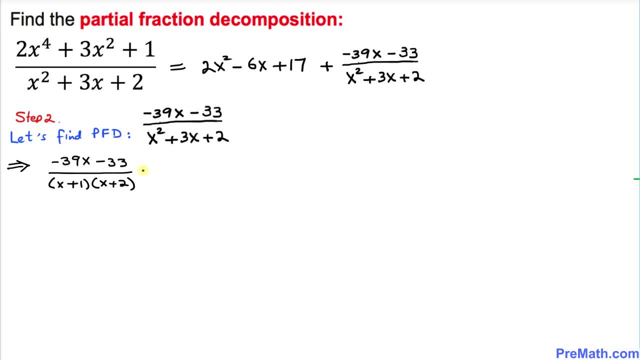 and since we have a, we have a, two linear factors at the denominator. so we are going to have two fractions, separated by plus sign. the first one is going to be x plus one, the other one is going to be x plus 2.. and the top we have a constant a for the first fraction and constant b for the. 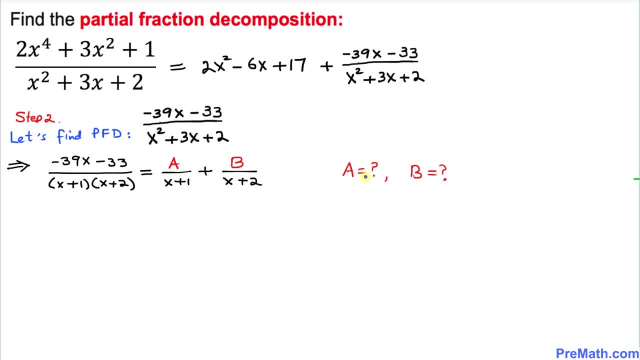 second fraction and we are going to find the value of these constant a and constant b. now, in our next step, let's focus on this denominator: x plus 1 times x plus 2. let's multiply this one across the board. so I'm going to multiply x plus 1 time x plus 2 on this left hand side, and now x plus 1 time. 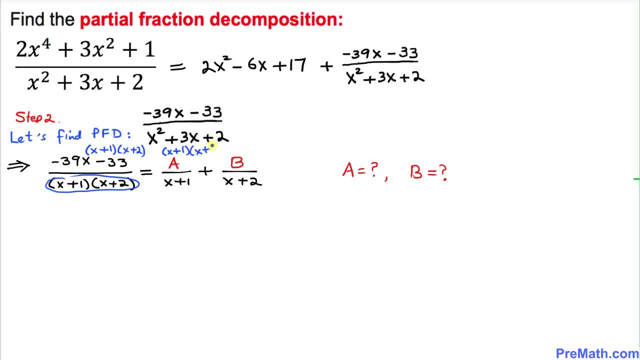 x plus 2 for the first fraction on the right hand side, and likewise x plus 1 time x plus 2 for the second fraction, and as we can see that these two linear factors cross out with this one, so we ended up with negative 39. x minus 33 on the left hand side equals to, as we can see, that this: 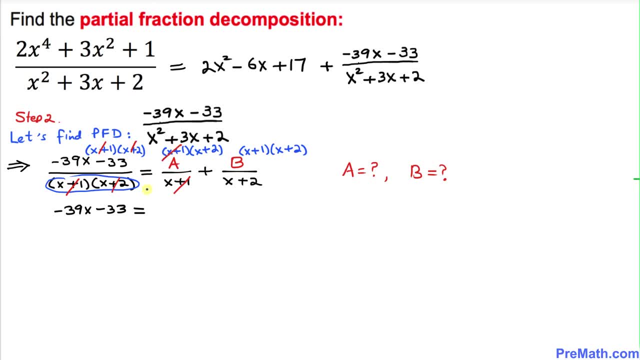 x plus 1 cancels out with this x plus 1, so we ended up with a times x plus 2, and likewise, on this side, this x plus 2 cancel with this x plus 2, so we ended up with plus b times x plus 1, and I am going to call this as an equation number 1. 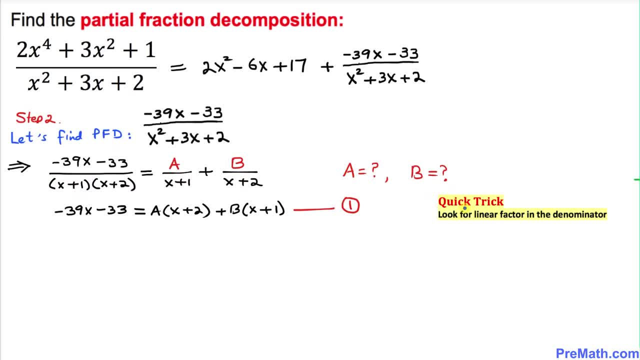 and here is our next step. we have a quick trick. look for linear factors in the denominator on this left hand side and, as we can see, we have a two linear factors. we are going to set them up equal to zero. so x plus 1, equal to zero, the first one. 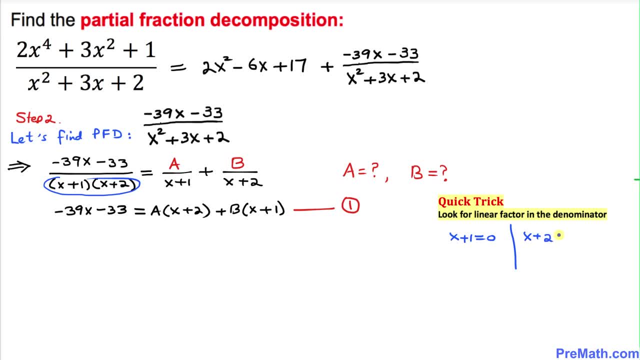 and let's set the second linear factor equal to zero as well. so our first value, x value, is going to be negative 1, and then second x value is going to be negative 2, and now let's focus on this: x equal to negative 1 value. 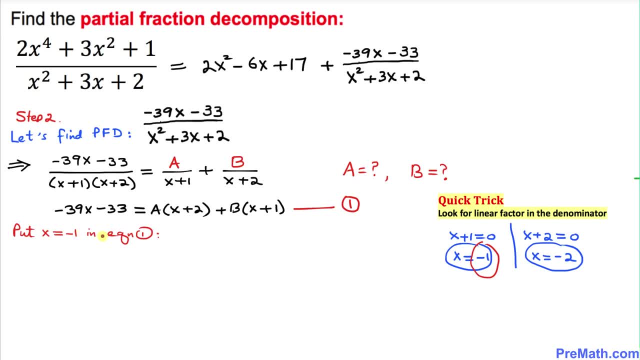 and I wrote down. put x equal to negative 1 value in this equation number 1. so wherever we see x, we are going to replace it by negative 1. so this left hand side is going to become negative 39 times negative 1 minus 33. 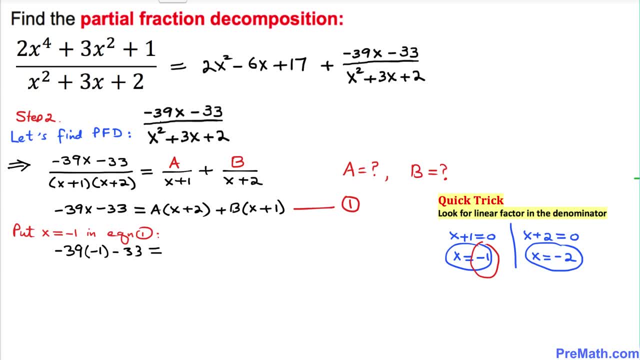 equal to, as we can see over here, this: when we replace this x by negative 1, so this negative 1 and positive 1 is going to give us zero. zero means this whole term is going to become zero. so let's go ahead and write down this. a by the way, a times x in our case, is negative. 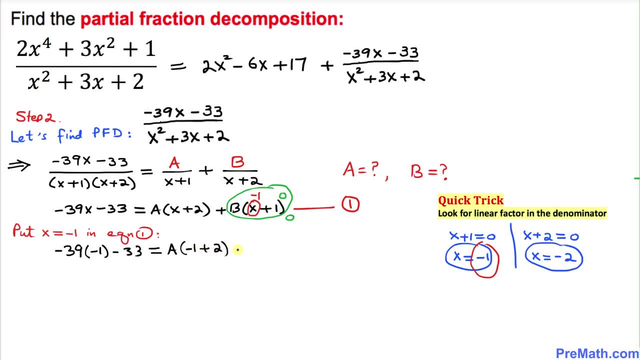 1 plus 2, and this thing we have zero. let's simplify, furthermore. so we are going to have, on this left hand side, positive 39 minus 33 equals to a times 1, which gives us a equal to 6 value. and now let's focus on 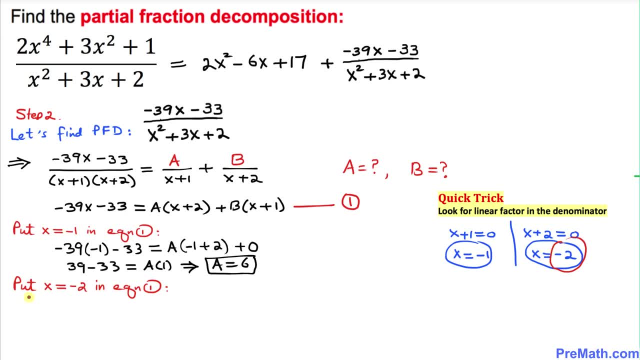 other value of x, which is negative 2, and here i wrote down: put x equal to negative 2 in this equation 1. that means wherever we see x, we are going to replace it by negative 2. so the left hand side is going to become negative 39 times negative. 2 minus 33 equals to: if we replace this: 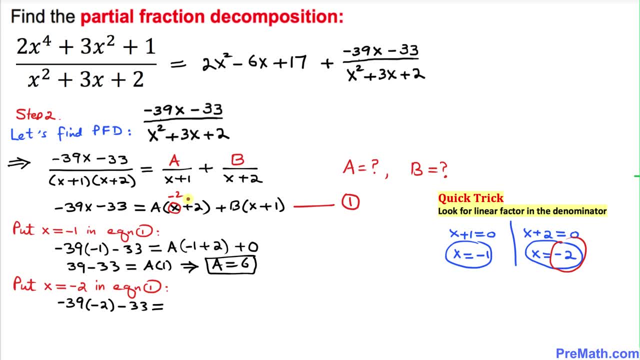 x by negative 2, negative 2 and positive 2 is going to give us 0, so 0 time whole thing is going to be 0. so i can write 0 on the right hand side plus b times. x is being replaced by negative 2 plus 1. let's simplify the left hand side. 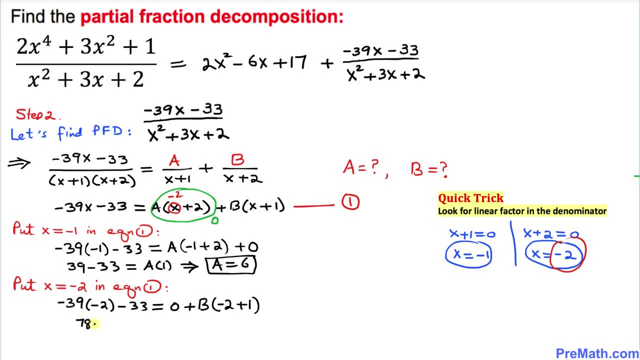 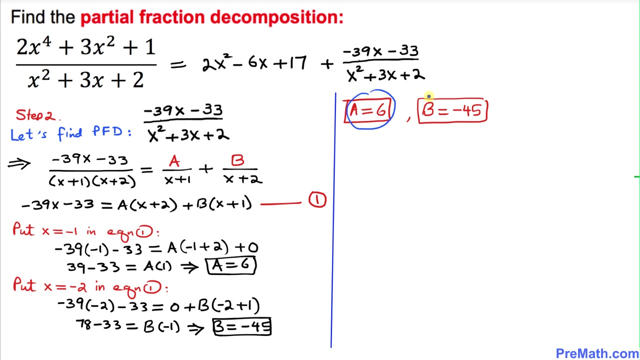 is going to be a positive 78 minus 33. equal to this is going to become b times negative 1. that means b value is going to be simply negative 1, 45. all right, so we got b value negative 45, so thus our a value turns out to be 6 and b value 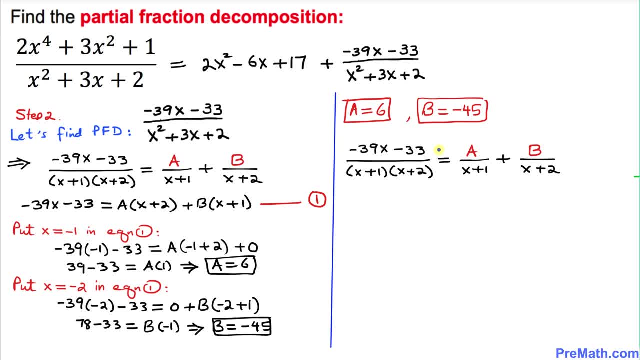 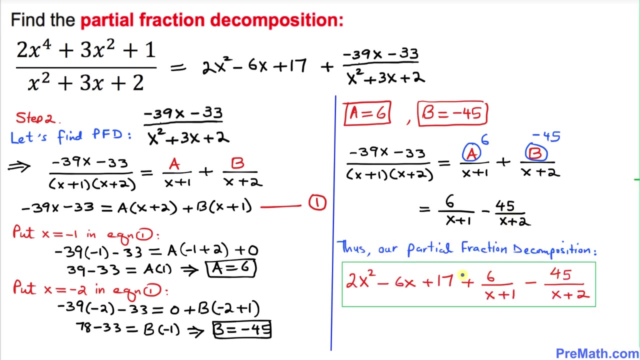 is negative 45 and therefore in our partial fraction decomposition, wherever we see a, we are going to replace it by 6 and b by negative 45. and here is our partial fraction decomposition, once we have replaced a by 6 and b by negative 45. thus our complete partial fraction decomposition.